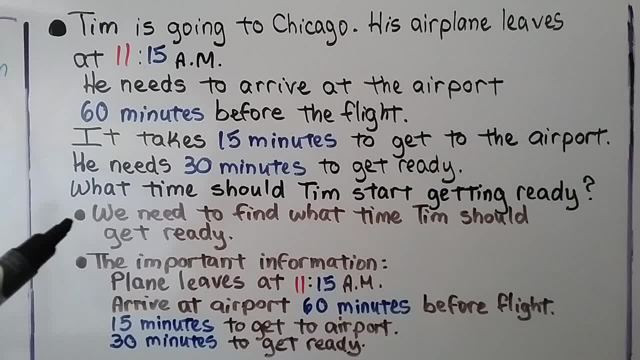 start getting ready. So we need to find what time Tim should get ready, And our important information is that the plane leaves at 11: 15 am. That's important, so we can underline that. What's also important is that he needs to arrive at the airport 60 minutes before the flight. We can. 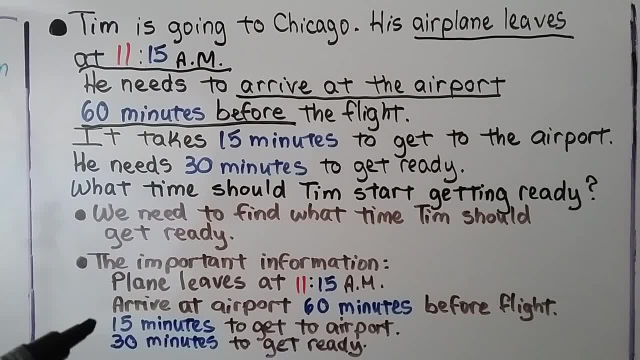 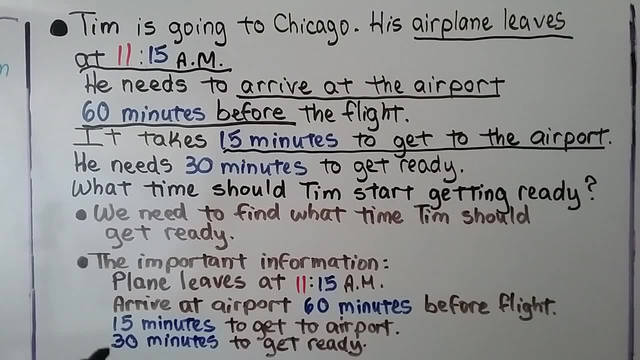 underline that. It is also important that he needs 15 minutes to get to the airport And we need to know that it's going to be 30 minutes to get ready. So we need to underline 30 minutes to get ready. So now we have collected all the important information in the word problem. 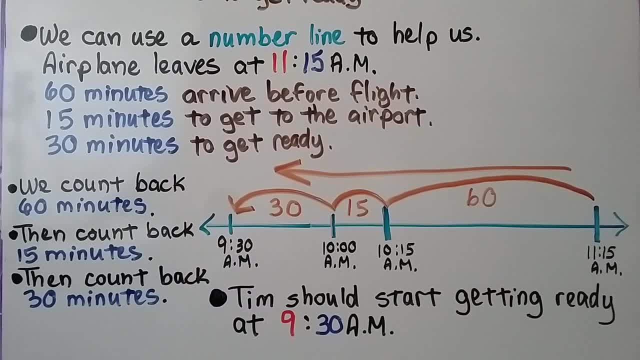 We can use a number line to help us. The airplane leaves at 11: 15 am. There's 60 minutes that he needs to arrive before the flight: 15 minutes to get to the airport and 30 minutes to get ready. What we do is because we know the airplane leaves at 11: 15. we need to find out when he gets ready, So we need to find the start time. 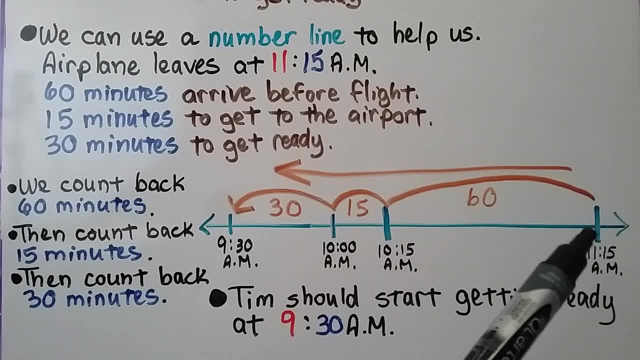 Our number line is going to go from 11- 15 am And we're going to skip count Backwards. We're going to skip by the elapsed time. So from 11- 15 am, 60 minutes is one hour. That'll put us at 10- 15 am. 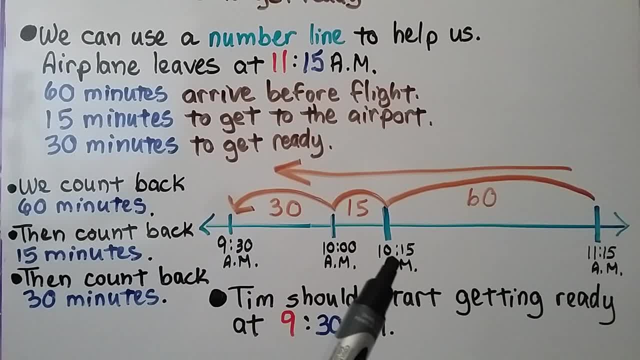 Then we need 15 minutes to get to the airport. So we're going to go back 15 minutes. That puts us at 10 am. Then he needs 30 minutes to get ready. We're going to skip 30 and we'll be back at 9: 30 am. 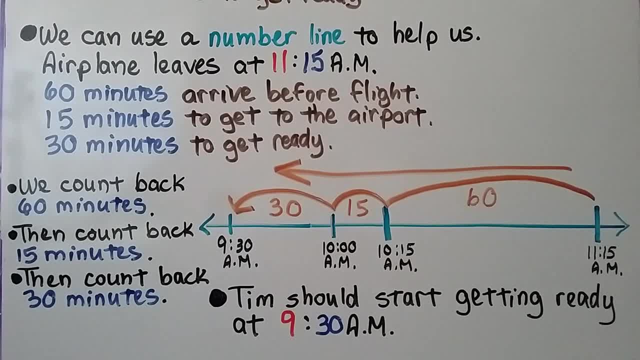 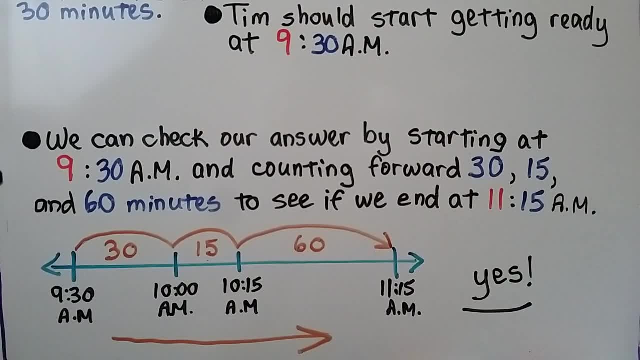 So we know Tim should start getting ready At 9: 30 am Or earlier, Right, And we can check our answer by starting here at 9: 30 and counting forwards the 30 minutes, 15 minutes and 60 minutes to see if we end at 11: 15 am. 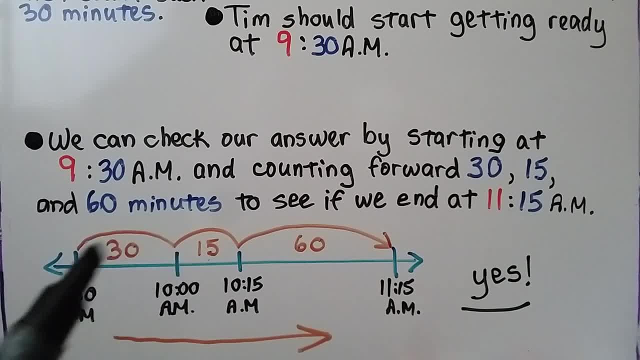 When his flight leaves. We go from 9- 30 to 10. that's 30 minutes. Then we add 15 more minutes, So we're at 10- 15.. We had 60 minutes is an hour And we get to 11- 15 am. 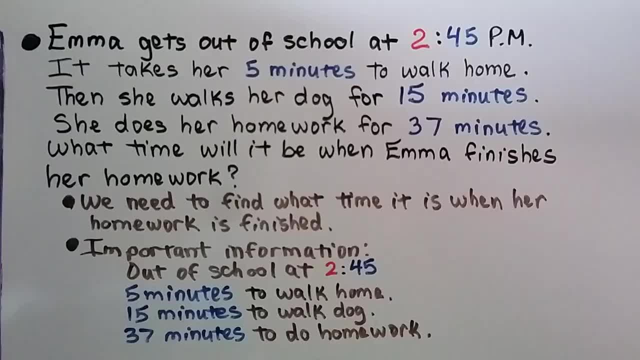 So yes, that worked. Emma gets out of school at 2: 45 pm. It takes her five minutes to walk home. Then she walks her dog for 15 minutes. She does her homework for 37 minutes. What time will it be when Emma finishes her homework? 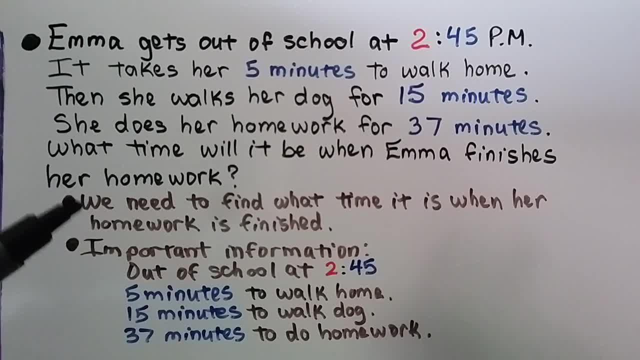 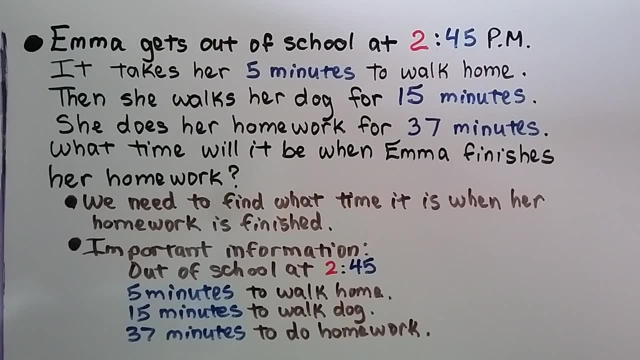 What do we need to find? We need to find what time it is when our homework is finished. The important information Is that she's out of school at 2: 45 pm. We can underline or circle that important information. It's also important that it takes her five minutes to walk home. 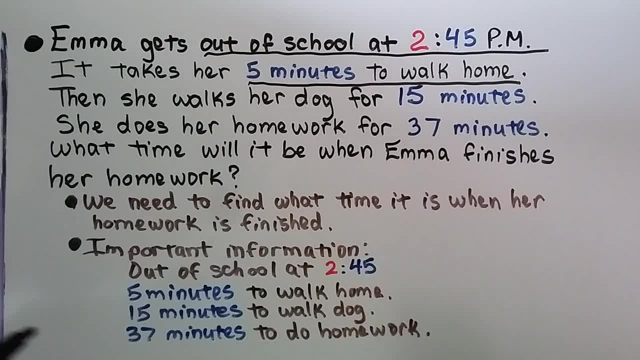 We can underline or we could circle that information. It's important that it's 15 minutes she spends walking the dog. We can underline that information. And it's important to know that it took 37 minutes to do her homework, So we can underline homework for 37 minutes. 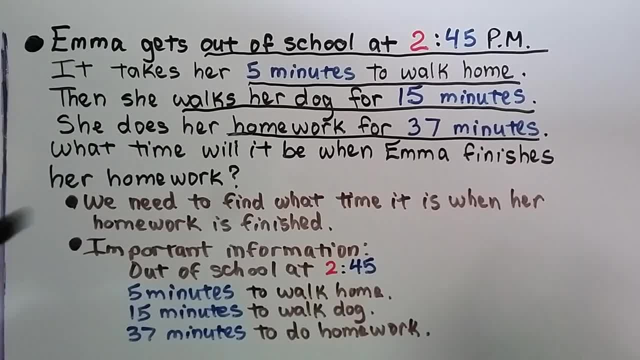 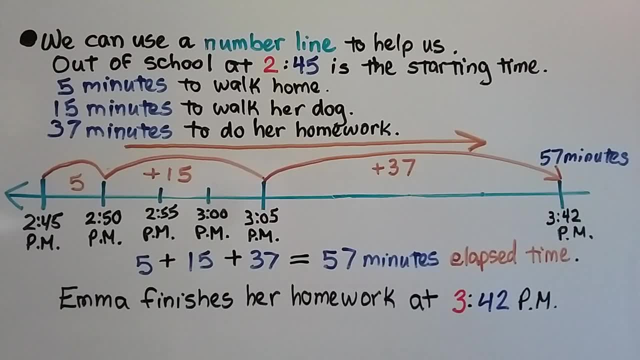 Now that we've gathered all our important information and we know what we need to find, We can start solving it. We can use a number line to help us. We know she's out of school at 2: 45.. That's going to be our starting time. 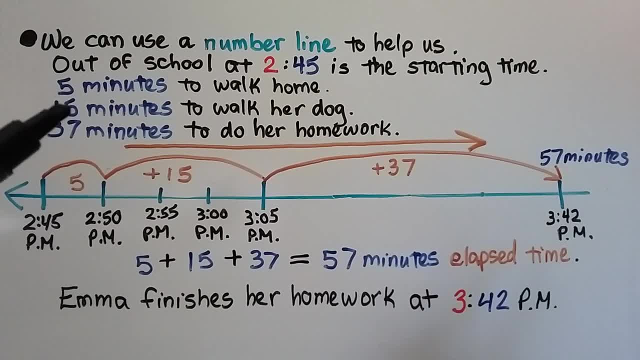 Then she has five minutes she walks home: 15 minutes to walk her dog and 37 minutes to do her homework. We need to find what time it is. When all of these things are finished, We start at our starting time: 2: 45 pm. 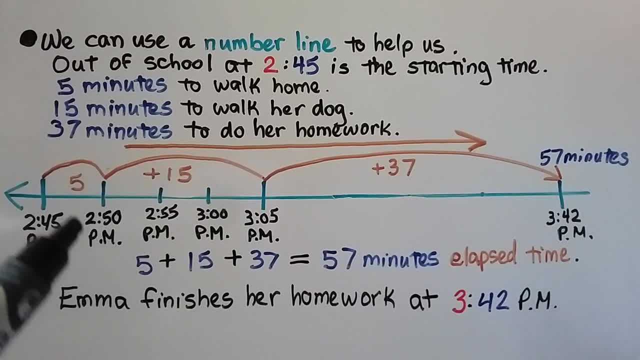 And we add five minutes for her to walk home. Now it's 2: 50 pm, Then we add the 15 minutes. We skip the 15 minutes that she walks her dog And going from 2: 50 pm. 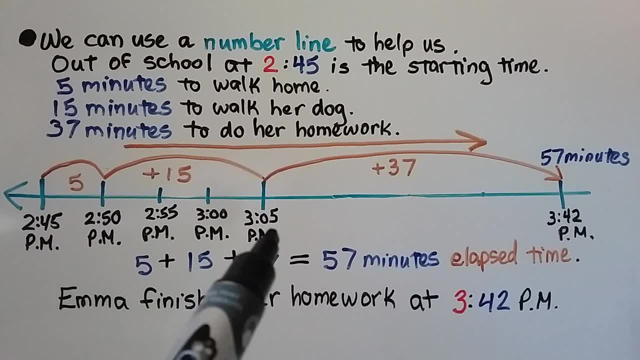 And doing 15 minutes, We've got five, 10, 15 minutes. That puts us at from 2, 50 to 2, 55. Then it becomes three o'clock, Then 3 0, 5 pm. So 15 minutes has us at 3, 0, 5 pm. 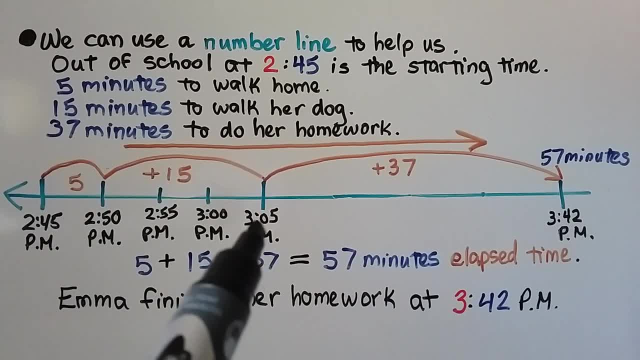 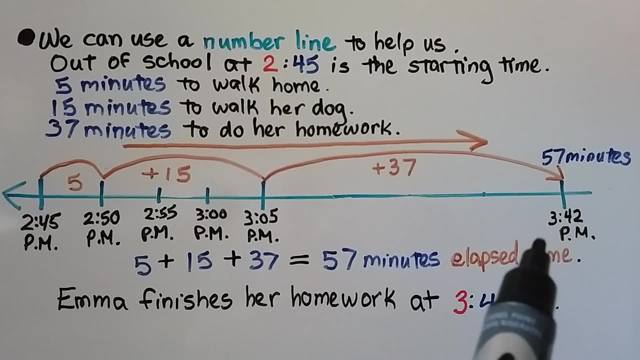 Then she does 37 minutes of homework. We need to add 37 minutes to 3: 0 5 pm. We skip 37 minutes And we're at 3: 42 pm Now. five plus 15 plus 37 is equal to 57.. 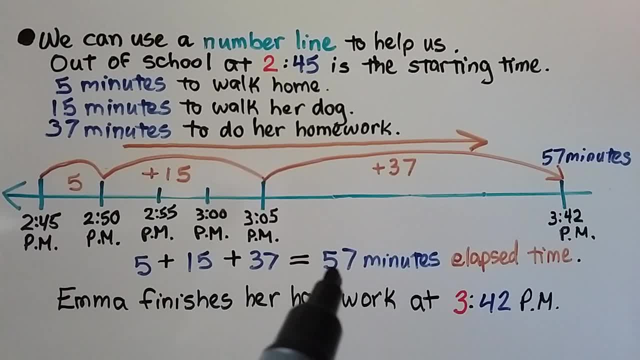 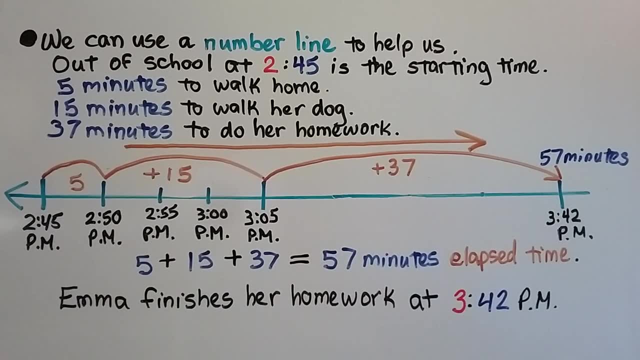 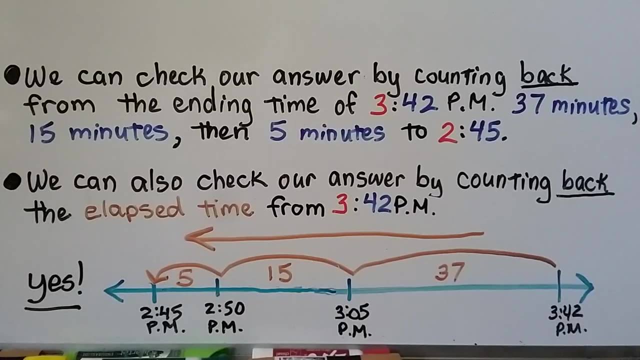 Five plus 15 is 20.. Plus the 37 makes it 57. So that's our total Of elapsed time. This whole thing should be 57 minutes. We know Emma finishes her homework at 3: 42 pm. We can check our answer by counting back from the ending time of 3: 42 pm. 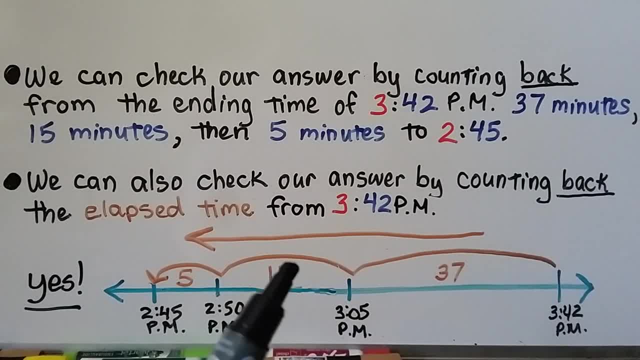 The 37 minutes, the 15 minutes and the five minutes back to 2: 45 pm. We can also check our answer by counting back the elapsed time, The entire 57 minutes From 3: 42 pm, And, yes, we will land at 2: 45 pm. 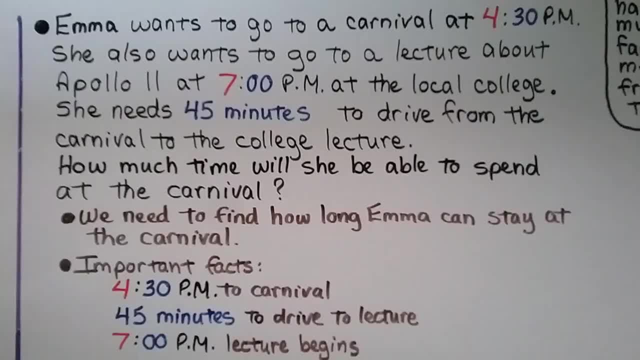 So we know we did it correctly. Emma wants to go to a carnival at 4: 30 pm. She also wants to go to a lecture about Apollo 11 at 7 o'clock pm At the local college. She needs 45 minutes to drive from the carnival to the college lecture. 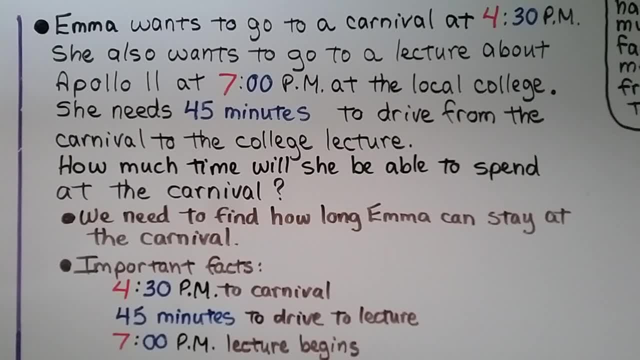 So how many minutes? So how much time will she be able to spend at the carnival? What do we need to find? We need to find how long Emma can stay at the carnival. The important facts are: she's going to be at the carnival at 4.30 pm. 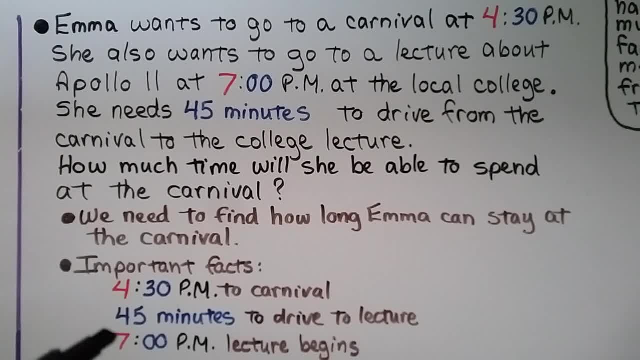 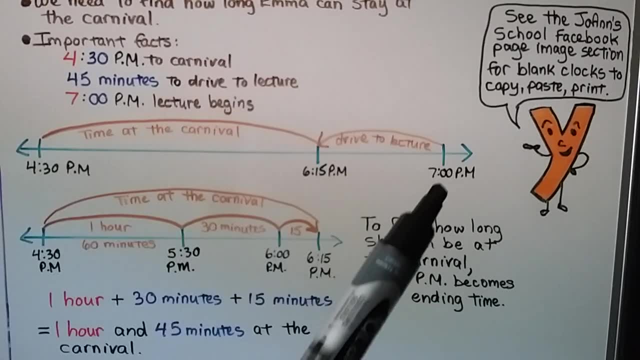 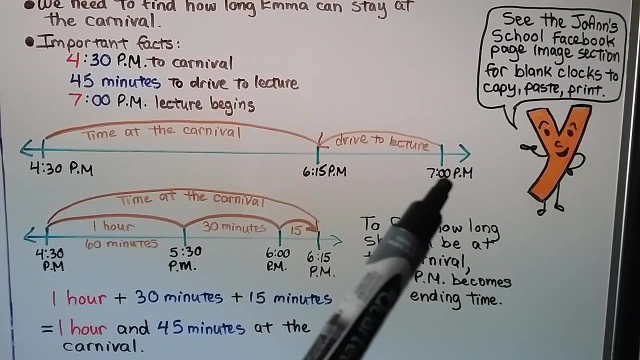 It takes 45 minutes to drive to the lecture and the lecture begins at 7 o'clock pm. We draw our number line and we know she needs to be at the lecture at 7 o'clock pm. We know it takes 45 minutes to drive to the lecture, so we start at 7 o'clock pm, our ending time, and we go back 45 minutes. 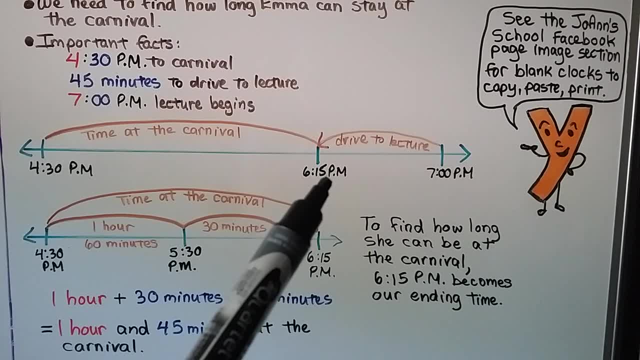 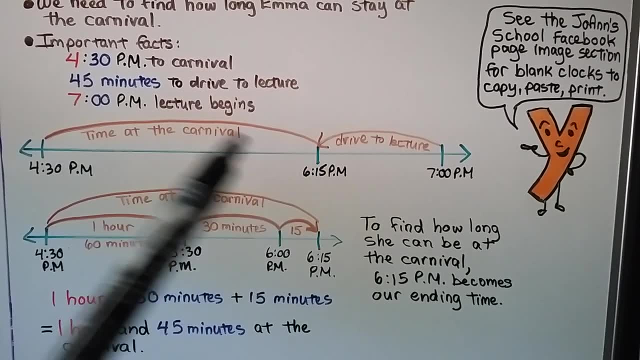 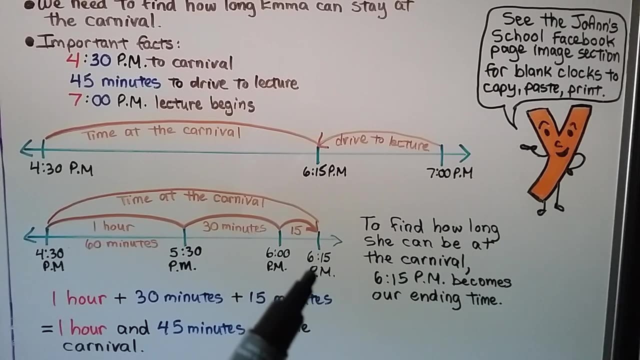 That's going to put us at 6.15 pm. Then the time between 4.30 pm and 6.15 pm is the time that she'll be able to spend at the carnival. So to find how long she can be at the carnival, 6.15 pm becomes our ending time. 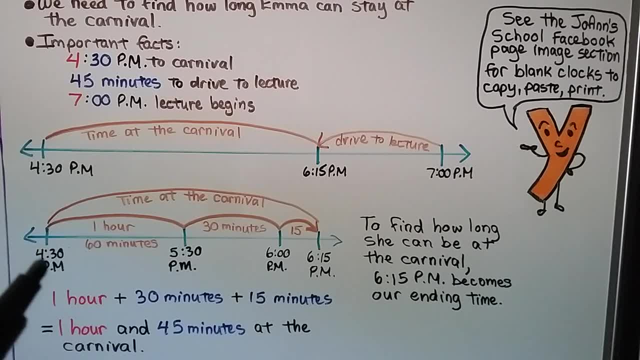 We draw our number line and we know that she's going to arrive at the carnival at 4.30 pm. If we go one hour forward from 4.30 pm, we'll be at 5.30 pm. 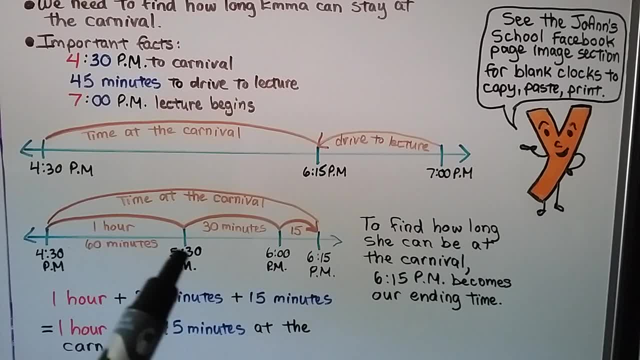 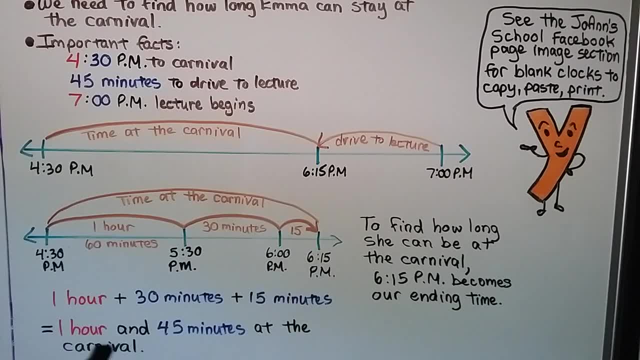 We went 1.30 pm to 6.15 pm. We went 1 hour plus 30 minutes plus 15 minutes. That's 1 hour and 45 minutes. So we know that Emma can stay at the carnival for 1 hour and 45 minutes. 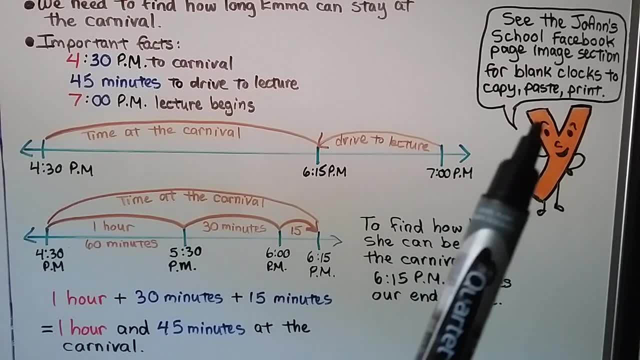 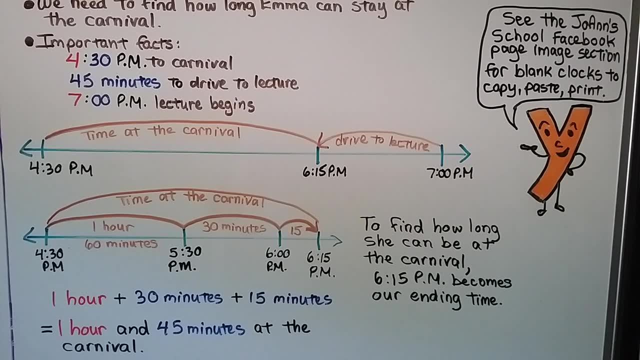 Now remember, you can go to my Facebook page in the image section and I've got blank clocks that you can copy, paste and print so that you can work with them. Bob got out of bed and ready for school. He spent 50 hours. 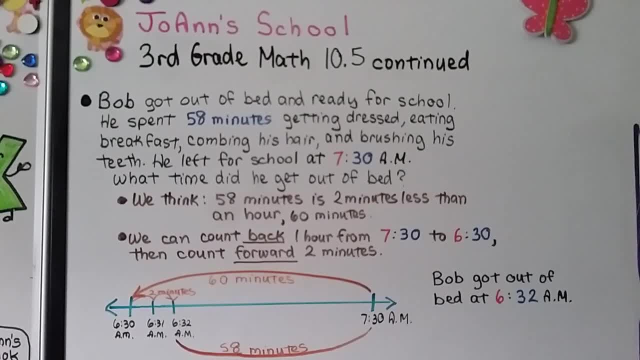 He spent 58 minutes getting dressed, eating breakfast, combing his hair and brushing his teeth. He left for school at 7.30 am, So what time did he get out of bed? What do we need to find? We need to find the time that he got out of bed in order to do these things for 58 minutes. 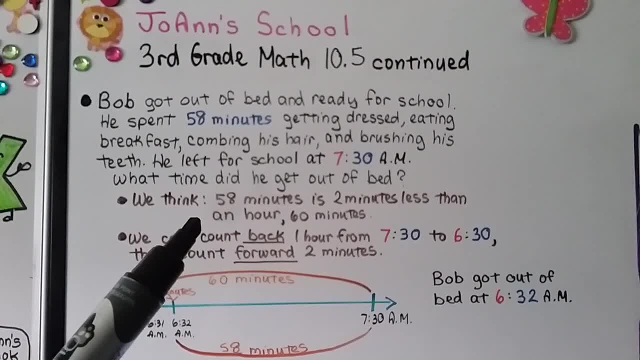 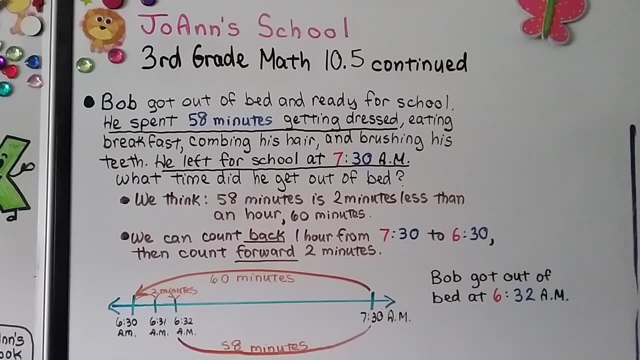 And we think 58 minutes is 2 minutes less than an hour 60 minutes. We need to underline the important information. It's important that he spent 58 hours 58 minutes getting dressed and getting ready and that he left for school at 7.30 am. 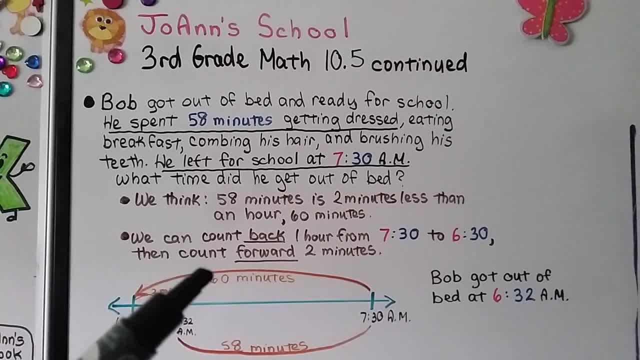 We can count back 1 hour, because 58 minutes is so close to an hour. We can count back from 7.30, when he left, to 6.30.. Then we can count forward 2 minutes, 1, 2.. 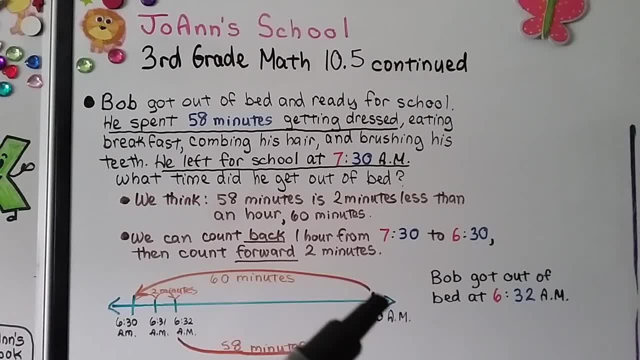 And that puts us at 6.32 am. From 7.30 back to 6.30 is 1 hour, but from 6.32 to 7.30 is 58 minutes. So we know, Bob. Bob got out of bed at 6.32 am. 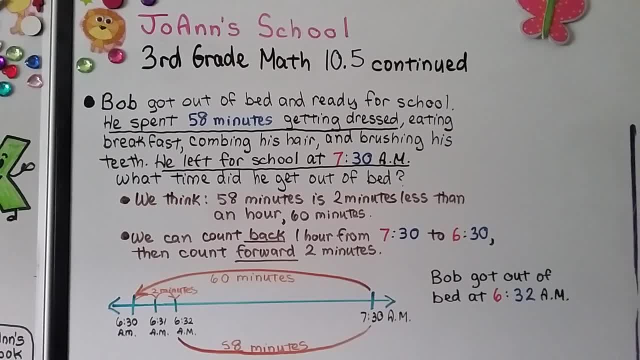 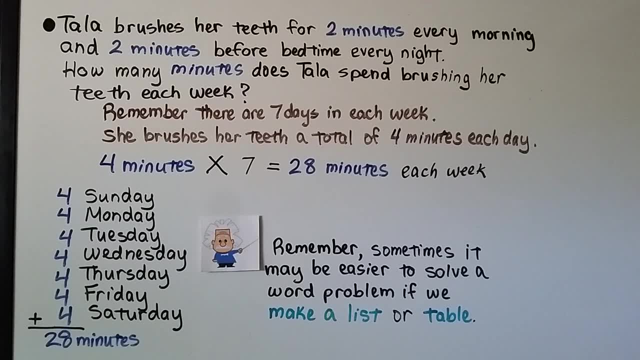 So we can use an hour to help us. Tala brushes her teeth for 2 minutes every morning and 2 minutes before bedtime every night. How many minutes does Tala spend brushing her teeth each week? So remember, there are 7 days in each week. 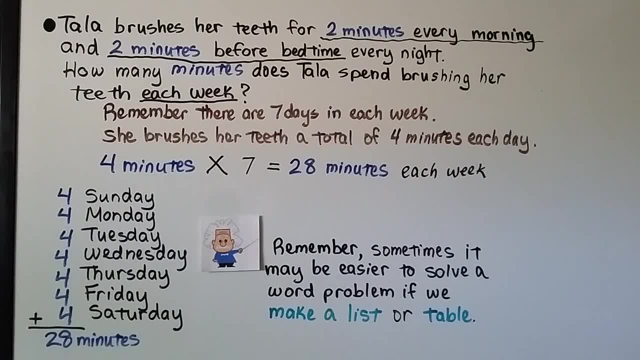 We need to underline the important information. It's important to know that she brushes for 2 minutes. So she says 4 minutes in the morning, 2 minutes before bedtime And they want to know how many minutes each week. So because she brushes her teeth, a total of 4 minutes each day. 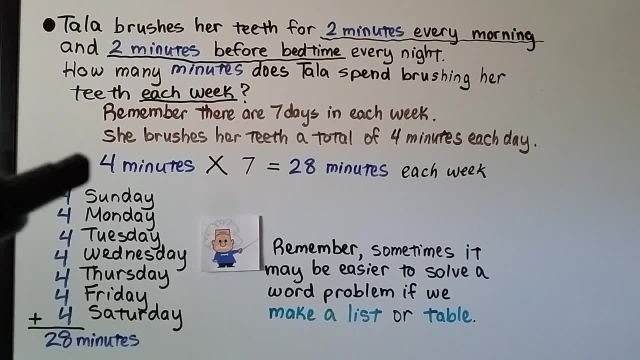 2 minutes in the morning and 2 before bed. We can do 4 minutes times those 7 days. 4 times 7 is equal to 28.. So she spends 28 minutes each week brushing her teeth. Now we can also write the days of the week. 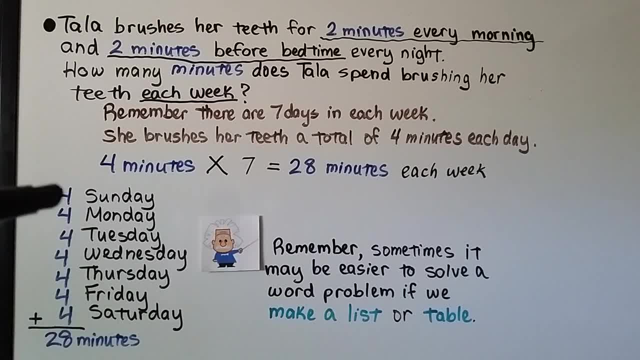 Sunday, Monday, Tuesday, Wednesday, Thursday, Friday, Saturday, and put a four for the minutes of each day that she brushes her teeth and we can add them up and we get 28 minutes. So remember, sometimes it may be easier to solve a word problem if we make a list or a table. 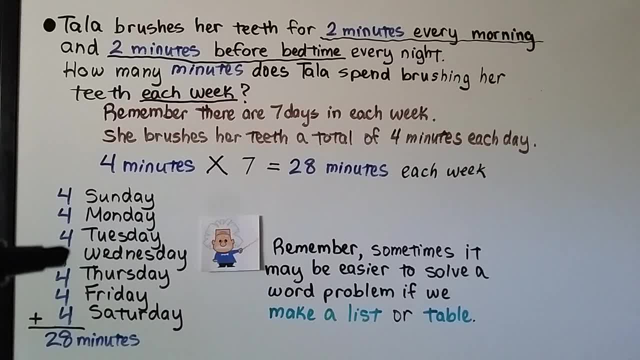 If we know she does 28 minutes a week, but it wanted to know how many minutes she brushed her teeth by Wednesday night. we would know that that's one, two, three, four days. That would be 16 minutes by Wednesday night when she went to bed. Okay, so you can make a list or table. 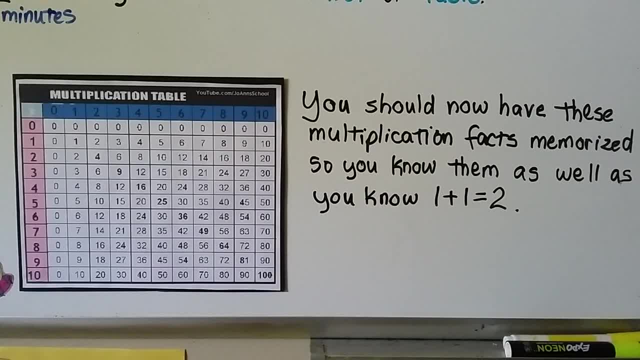 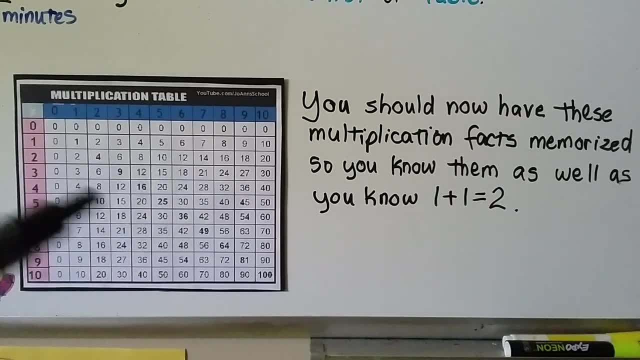 if that'll help you. So here's a multiplication table. We can do any number times any number, and here's the products. You should have these multiplication facts memorized by now. You should know them as well as you know that one plus one equals two. 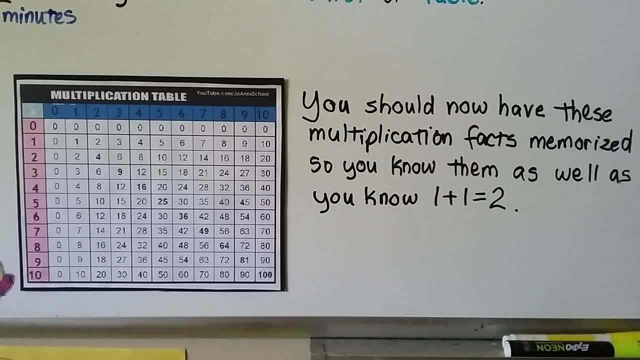 You should know them that quickly and students- people who memorize their multiplication table- do better at math. They have it easier at math as they get older and go on to higher grades. So to help yourself, make sure you have this multiplication table memorized.